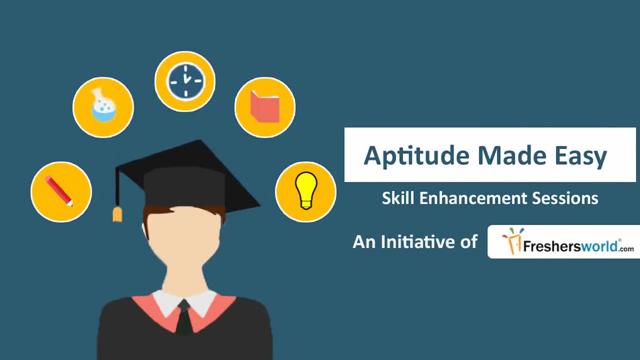 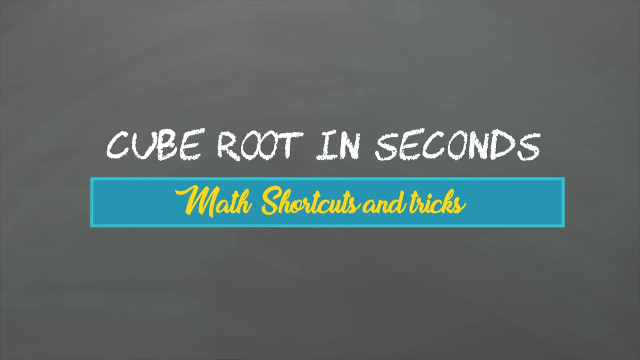 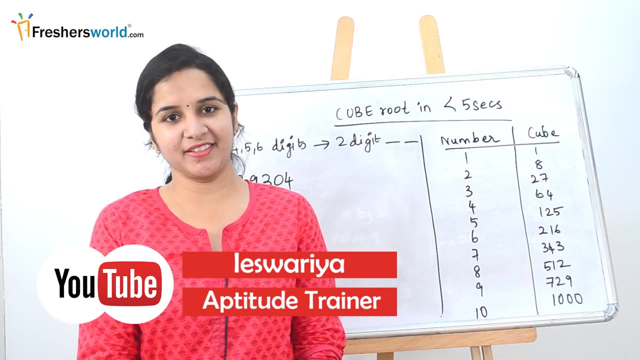 Hi friends, this is Aishwarya from Freshersworldcom. Welcome to our YouTube channel on Jobs and Careers. The topic that we are going to look today is how to find a cube root of a number in less than 5 seconds. 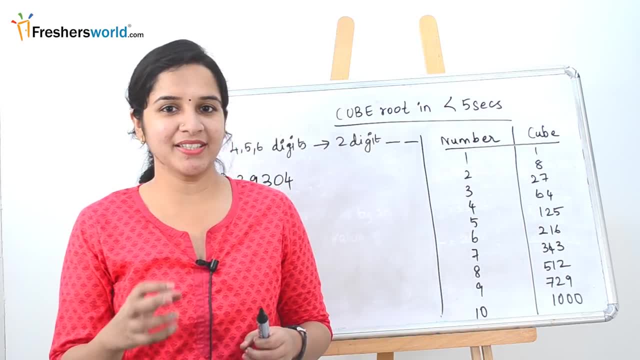 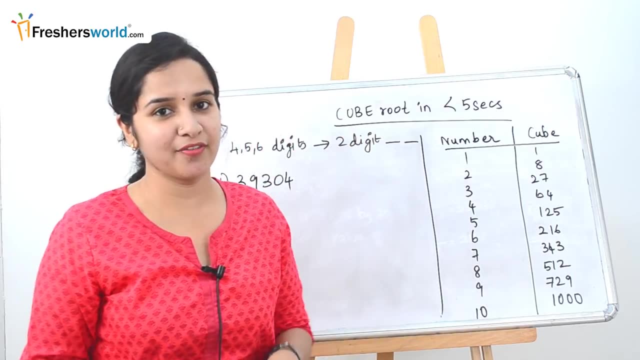 So how to find it? For that you have to make a little effort to understand the cube of all the numbers from 1 to 10. You have to definitely buy heart it to find the cube root in less than 5 seconds. It's very easy to remember this. One thing: you have to find it here that if you see all the unit digit 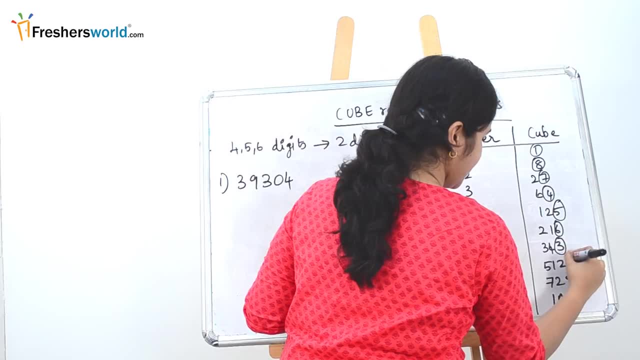 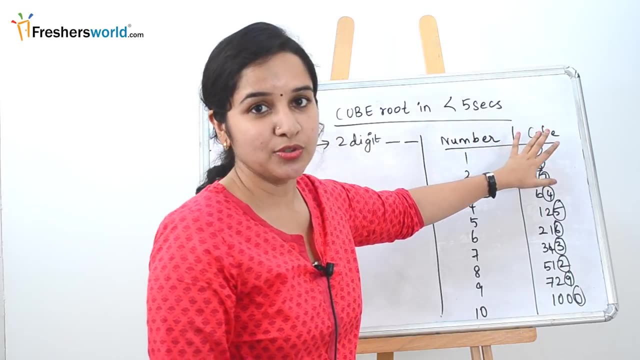 1,, 8,, 7,, 4,, 5,, 6,, 3, 2.. You can see from 0 to 9. all the numbers are being displayed in the cube. We will know its use while solving the sum. So another main thing that you should know is that 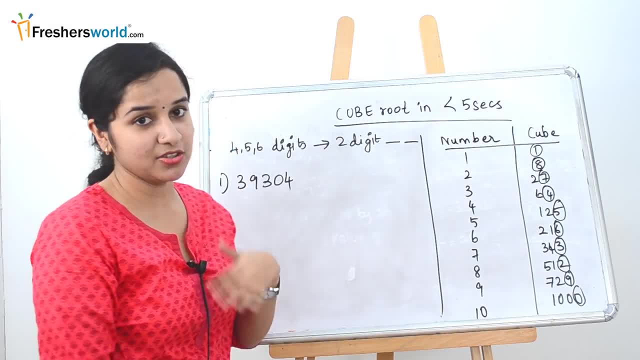 let's say, a digit that they have given in the question is a 4 digit or a 5 digit or a 6 digit? Always, your answer will be in a 2 digit. You have to just remember this. So let's start solving the sum. 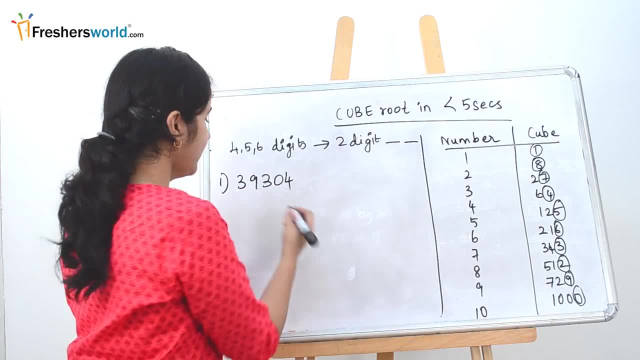 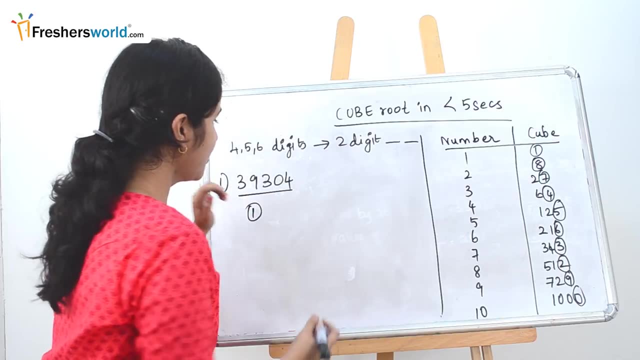 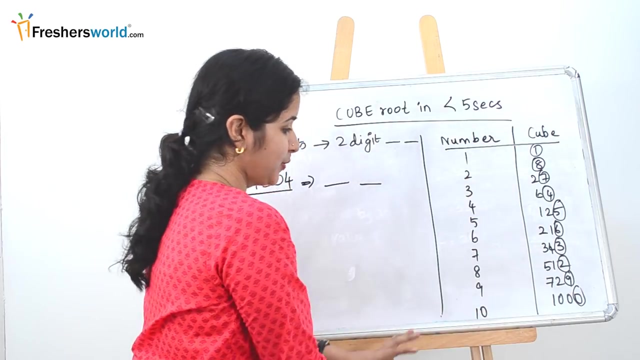 So the question that they have given is you have to find the cube root of 39304.. There are just only two steps to understand it. First step is: what is the unit digit here? It's nothing but 4.. So here first write it here from 1 to 10.. So unit digit is nothing but is 4.. 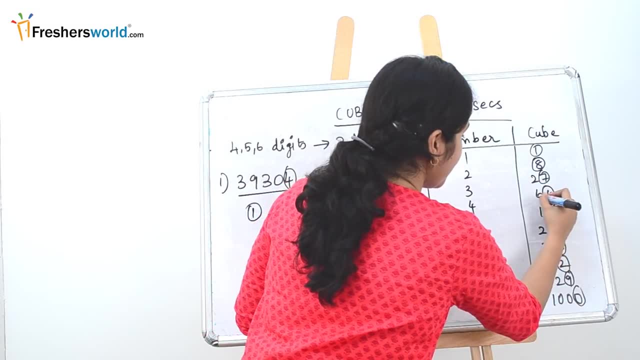 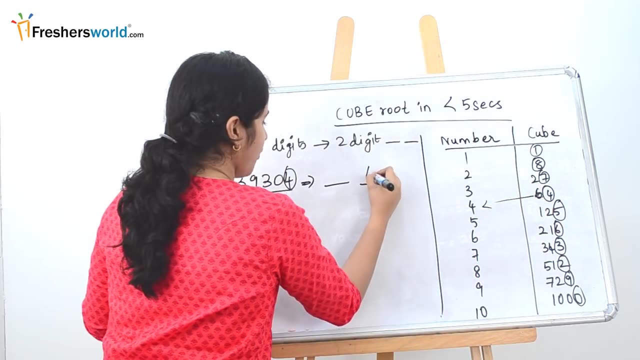 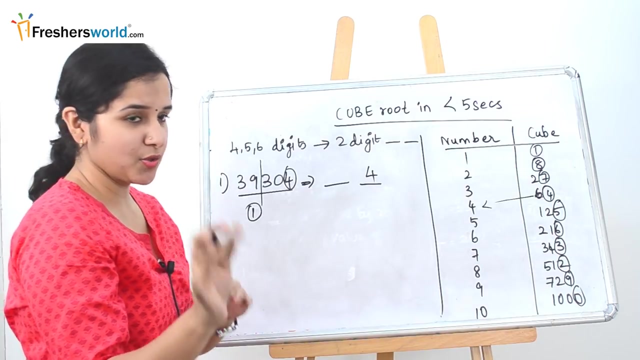 So find the number in which it ends in 4.. So you can see 64 here. it ends in 4.. The corresponding number to it is nothing but 4.. So write the 4 here directly. Next we have to omit the last 3 digits. So omit the last 3 digits: 304.. Take the first: 2.. It's 39.. 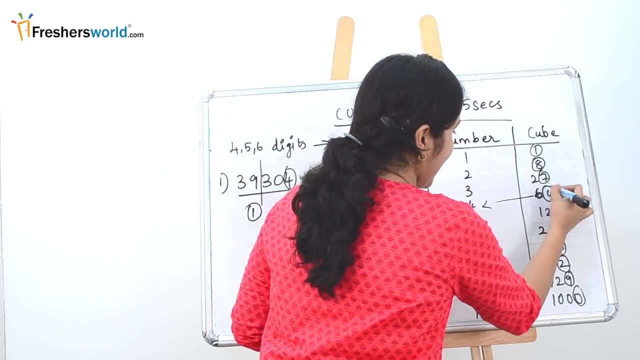 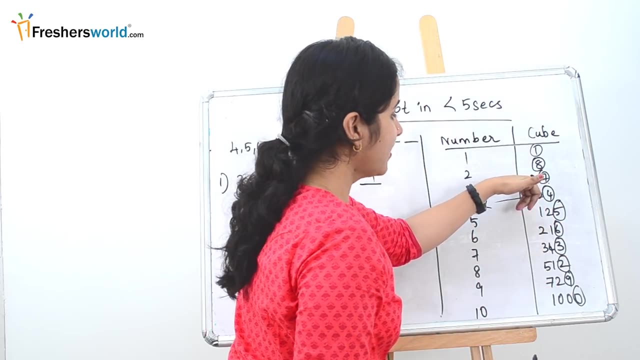 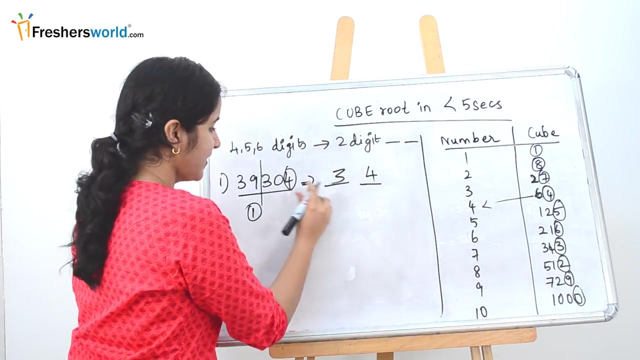 So 39 falls between 27 and 64. Find the smallest of it. So 27 is the smallest between 27 and 64. Write the corresponding number, which is nothing but 3.. So this is it. So what did we do? First, we take the unit digit and take the corresponding number to it. 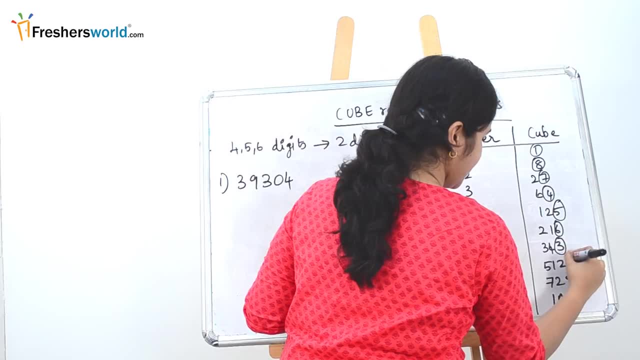 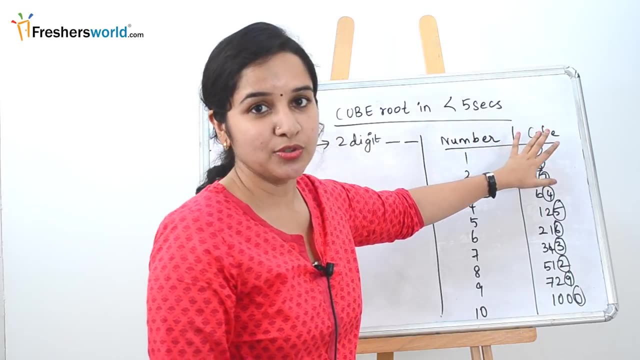 1,, 8,, 7,, 4,, 5,, 6,, 3, 2.. You can see from 0 to 9. all the numbers are being displayed in the cube. We will know its use while solving the sum. So another main thing that you should know is that 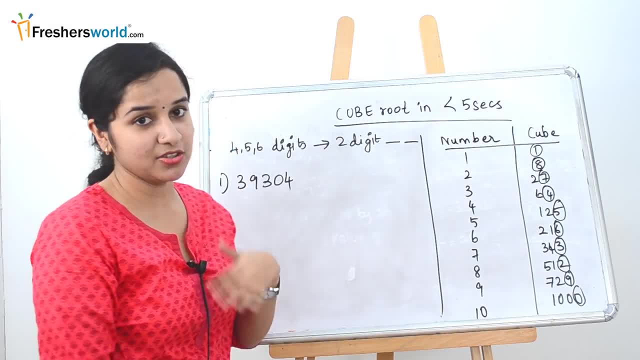 let's say, a digit that they have given in the question is a 4 digit or a 5 digit or a 6 digit? Always, your answer will be in a 2 digit. You have to just remember this. So let's start solving the sum. 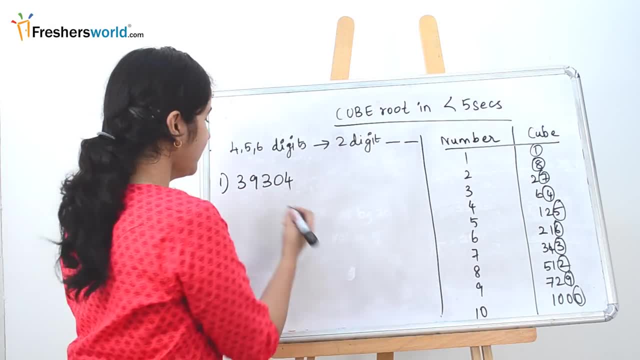 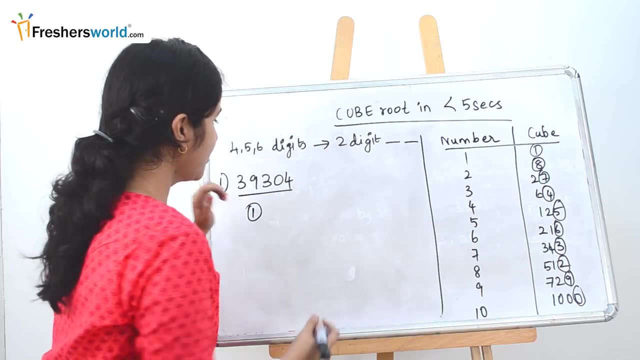 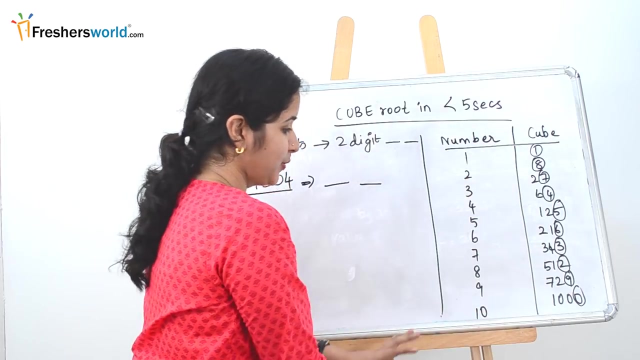 So the question that they have given is you have to find the cube root of 39304.. There are just only two steps to understand it. First step is: what is the unit digit here? It's nothing but 4.. So here first write it here from 1 to 10.. So unit digit is nothing but is 4.. 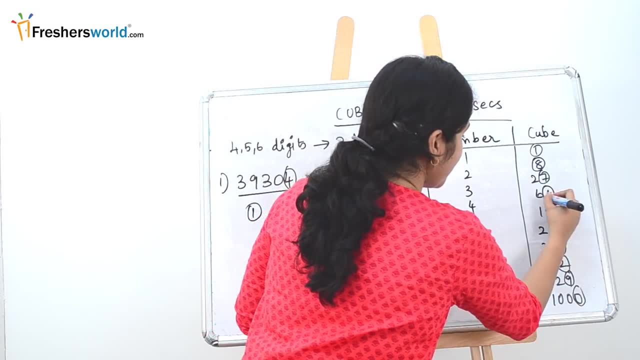 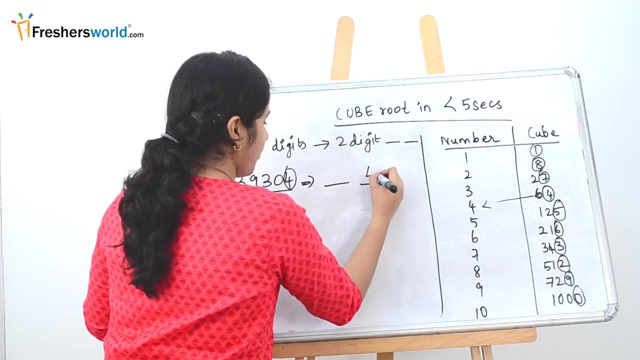 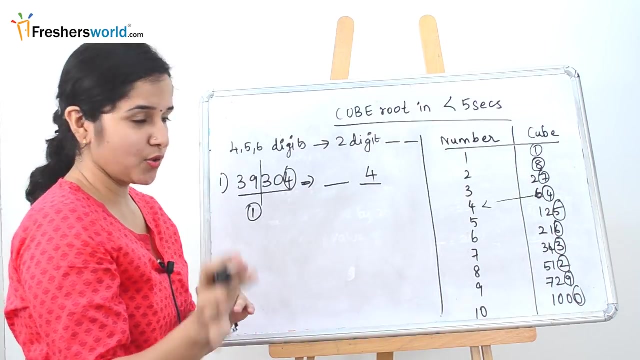 So find the number in which it ends in 4.. So you can see 64 here. it ends in 4.. The corresponding number to it is nothing but 4.. So write the 4 here directly. Next we have to omit the last 3 digits. So omit the last 3 digits: 304.. Take the first: 2.. It's 39.. 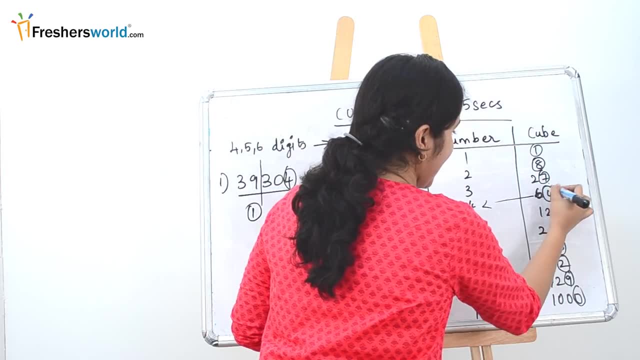 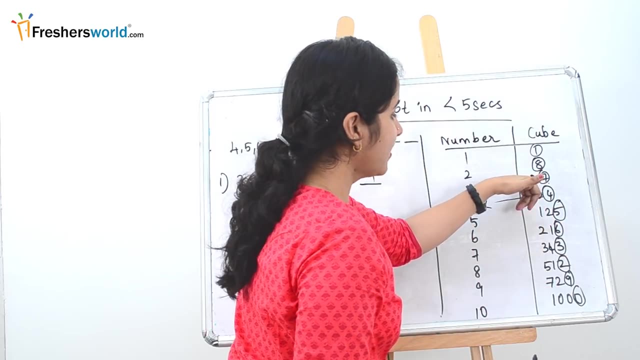 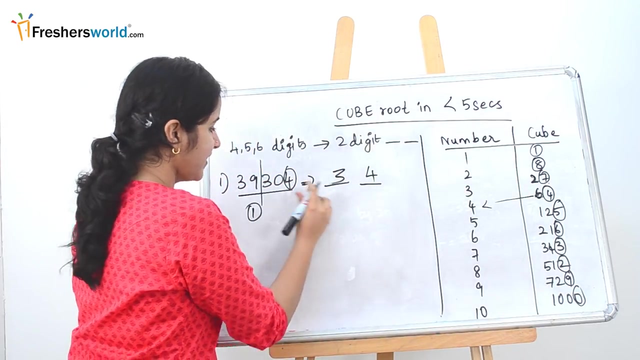 So 39 falls between 27 and 64. Find the smallest of it. So 27 is the smallest between 27 and 64. Write the corresponding number, which is nothing but 3.. So this is it. So what did we do? First, we take the unit digit and take the corresponding number to it. 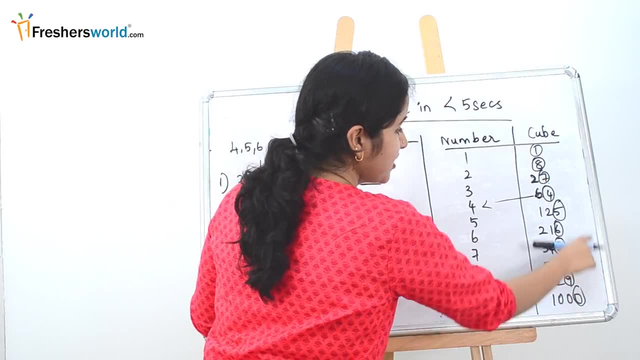 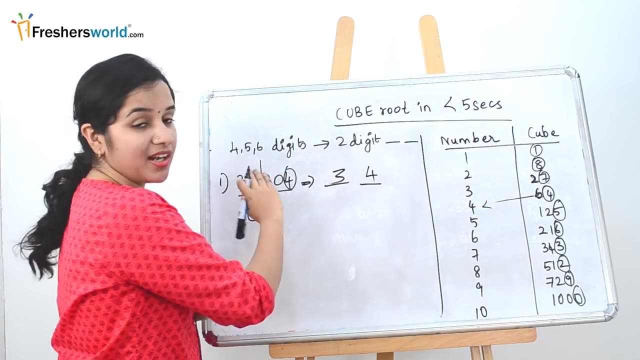 So unit digit is 4.. So find the number in which ends with 4.. This is 64.. The corresponding number to it is 4.. Directly write it. Second thing: what we did, We omit the last 3 digits. We took the first, 2.. First 2 is nothing but 39.. 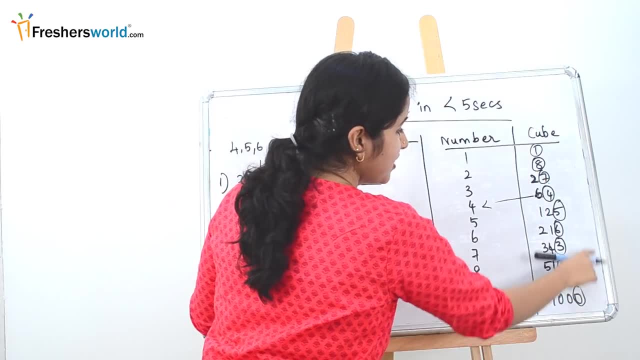 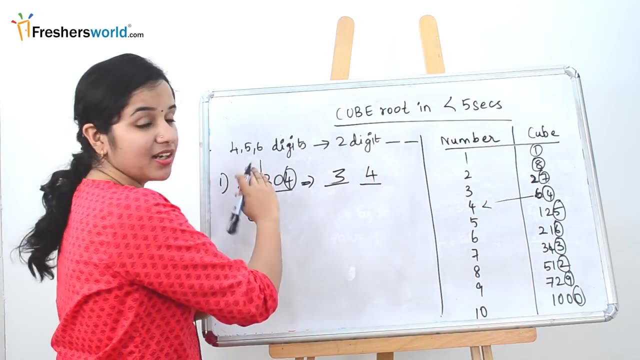 So unit digit is 4.. So find the number which ends with 4.. This is 64.. The corresponding number to it is 4.. Directly write it. Second thing: what we did, We omit the last three digits. We took the first, 2.. First, 2 is nothing but 39.. 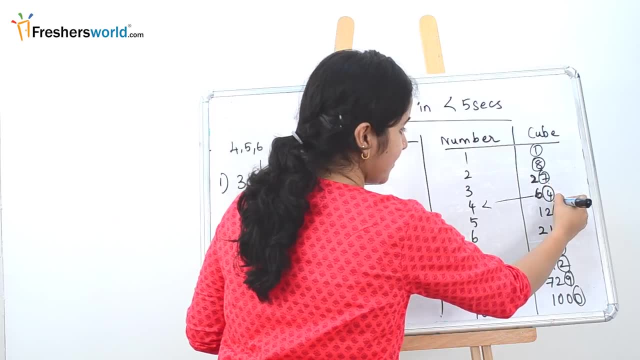 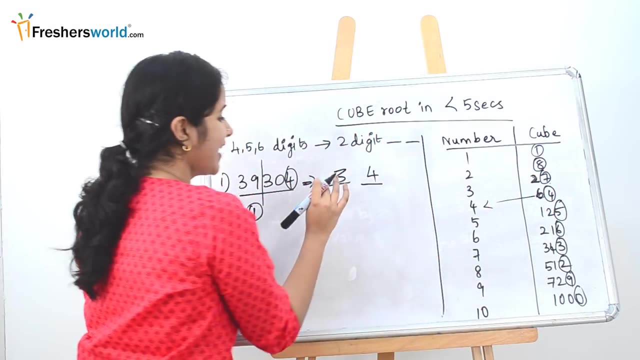 39 falls between the window of 27 and 64. Which is the smallest of it, 27.. So take 27 and the corresponding number to it, which is 3. So directly write it as 34.. Let's solve a couple of problems to understand this concept much better. 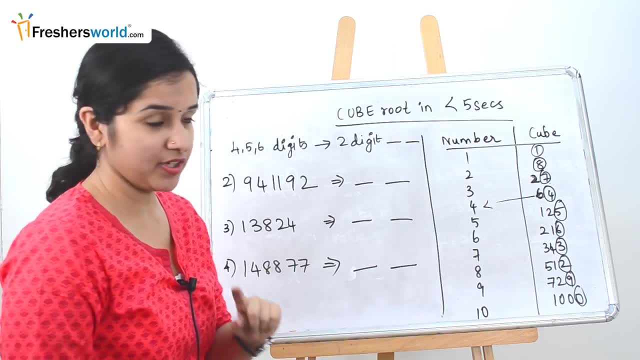 The second sum is that they have given 94,, 1,, 1,, 9,, 2. First step, So you have to take 2.. So 2 ends at 8.. So put the 8 here directly. 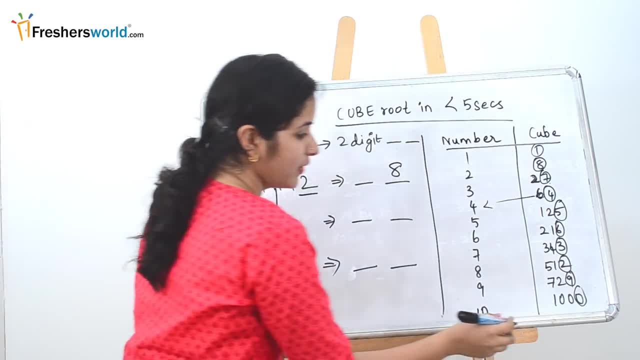 Omit the last. 3. Take the 9, 4, 1.. So 9, 4, 1 falls between 7, 29 and 1000.. With smallest 1 is nothing but 9.. So directly write 98.. 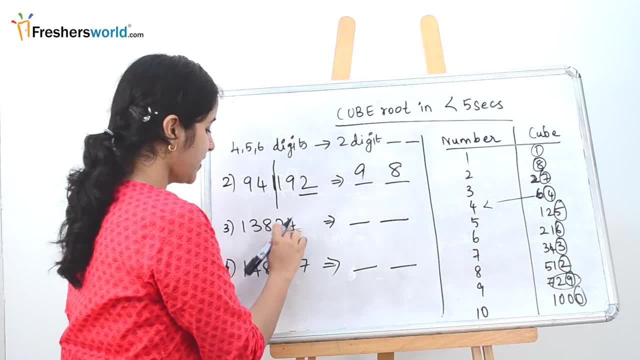 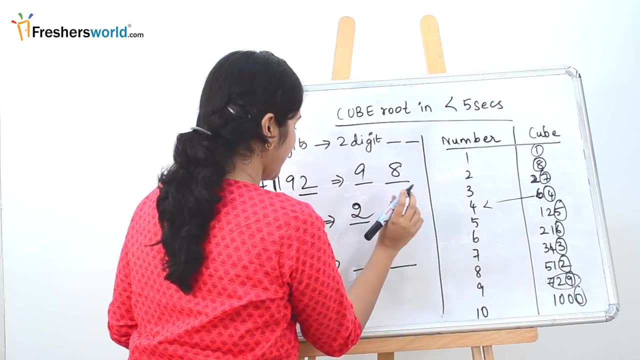 Let's see how I am going to solve the 3rd and 4th Within seconds. So here, 4 falls under number 4. Then run with 8 to 4. And 13 falls between 18 and 27, which is nothing but 24.. 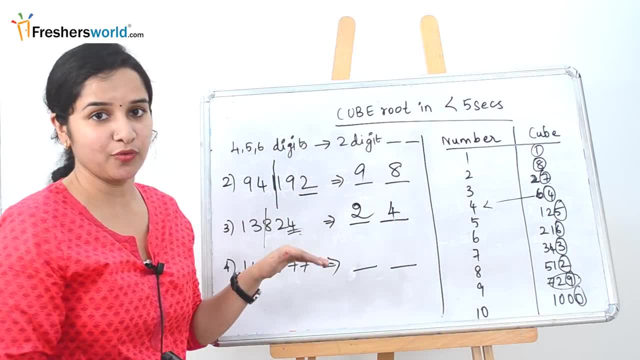 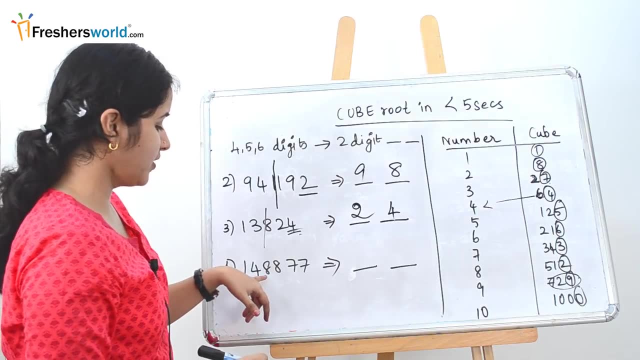 So you can see that how easily I solved for 138 and 24.. It's directly nothing but 24.. Let's see how I am going to solve it for the same thing, which is for a 6 digit number. It is 148877.. 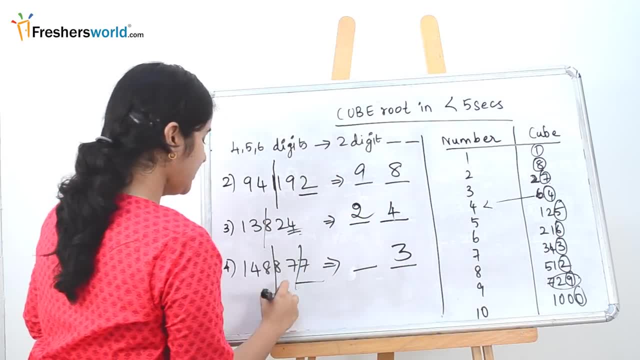 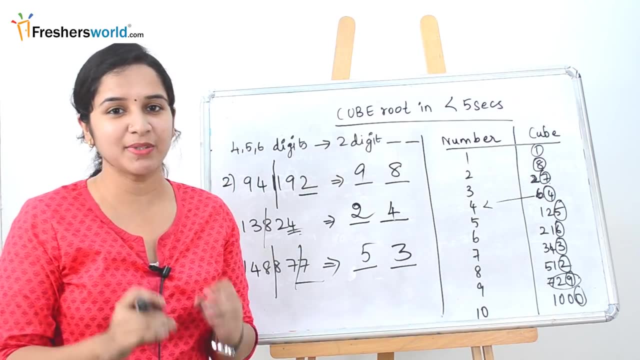 7 falls between: 3. Omit the last- 3. 5. So you see how easily we are able To find the cube root of a number: within split seconds. To find the cube root in less than 5 seconds. 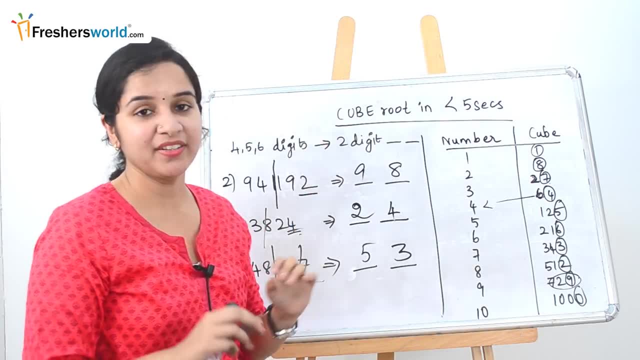 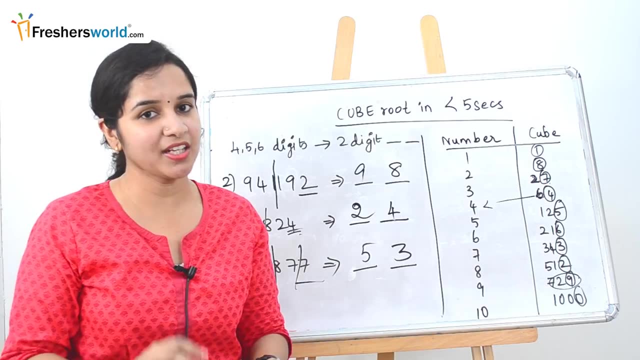 Two things you have to do. One is you have to know the cube from 1 to 10 very thoroughly And then follow the steps that we have discussed today in the cube root problem. If you know these two things, it will be very easy for you to find the cube root in less than 5 seconds. 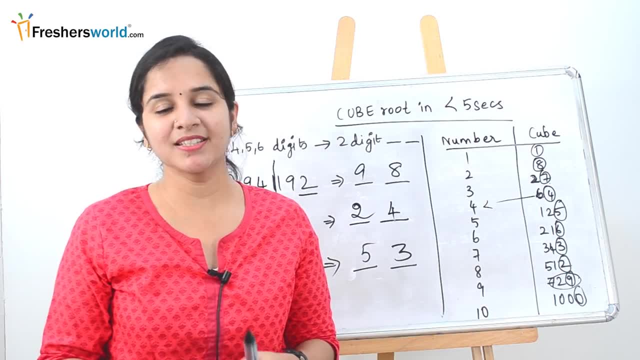 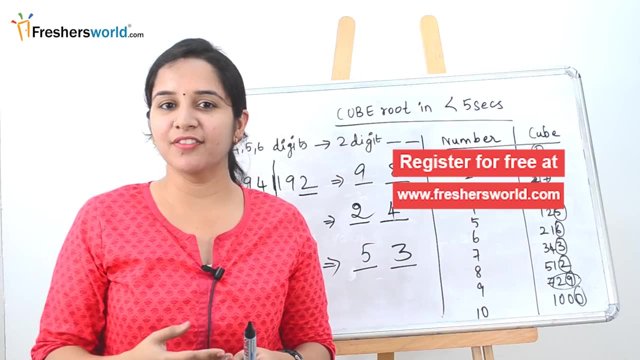 So in the upcoming videos we will be discussing on the various matrix which you can utilize in an aptitude exam to solve your sum very easily. So if you are a person who is looking for a job, kindly register in our freshersworldcom. 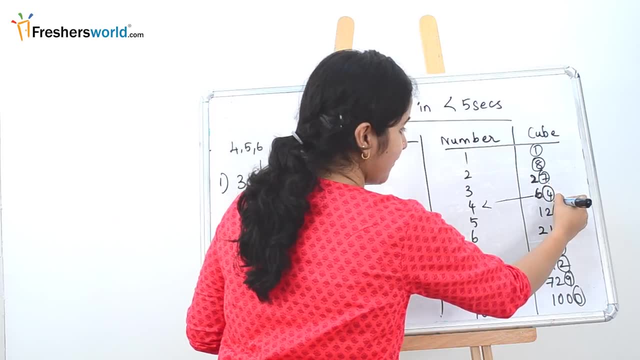 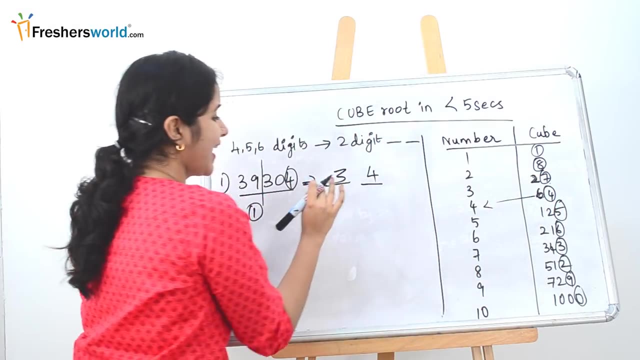 39 falls between the window of 27 and 64. Which is the smallest of it, 27.. So take 27 and the corresponding number to it is 3. So directly write it as 34.. So let's solve a couple of problems to understand this concept much better. 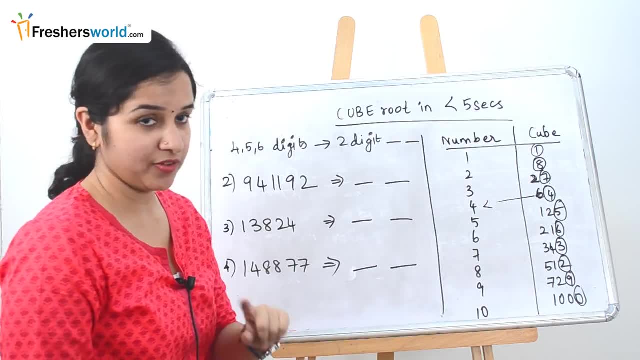 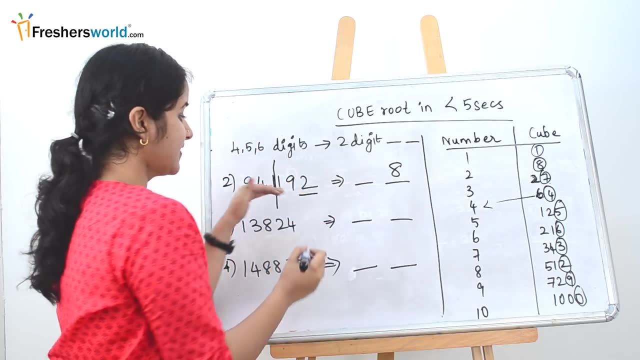 The second sum is that they have given 941192.. First step, So you have to take 2.. So 2 ends at 8.. So put the 8 here directly. Omit the last. 3. Take the 941.. 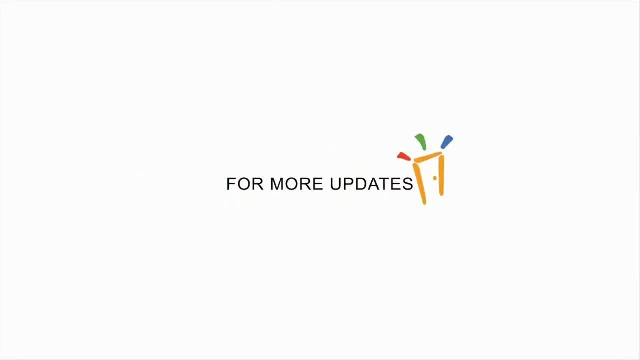 Like this video and subscribe to our channel. Thank you, Thank you.